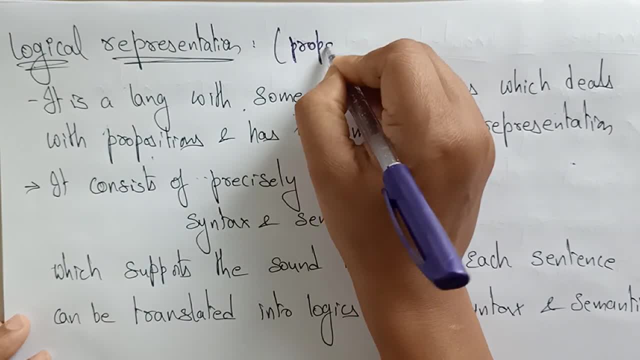 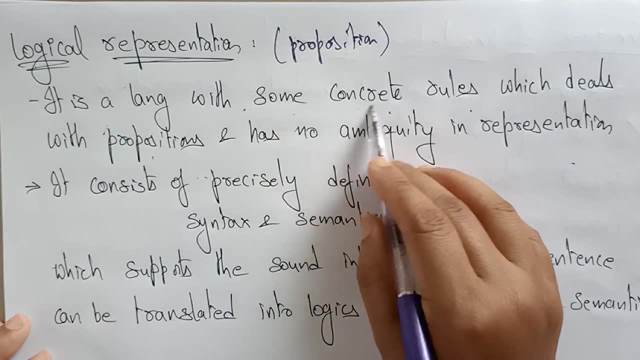 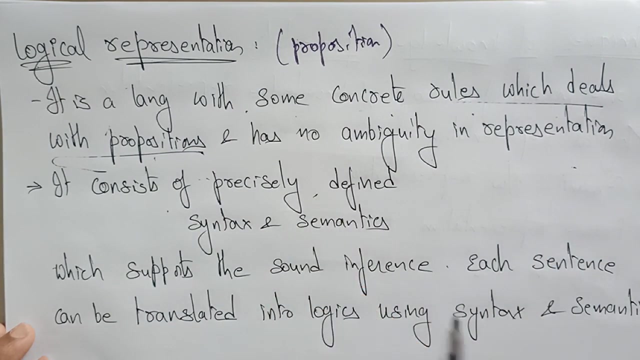 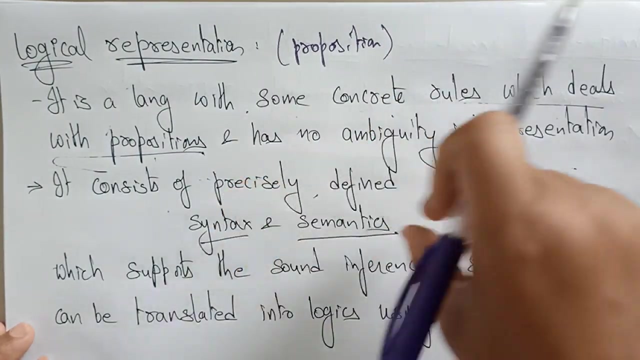 is you dealing with the propositions? With the help of the propositions, you're going to create some logical rules which deals with the propositions and it has no ambiguity in representation also, And it consists of preciously defined in syntax and semantics. The logical representation can be represented in the syntax and semantics. So which supports 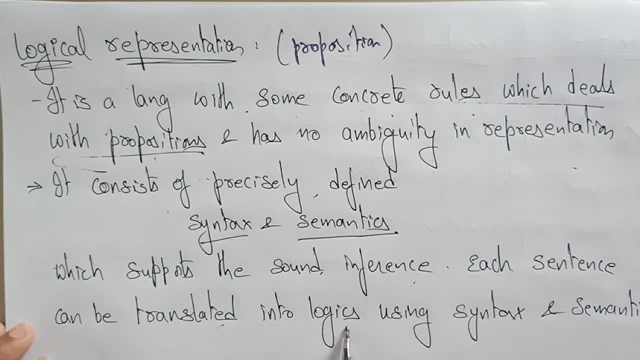 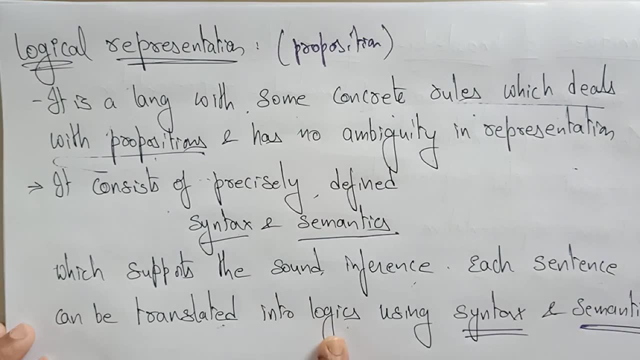 the sound inference. Each sentence can be represented in the syntax and semantics. It can be translated into logics using syntax and semantics. Whatever the sentence that is a knowledge sentence is there that can be translated into logics using syntax and semantics. Okay so. 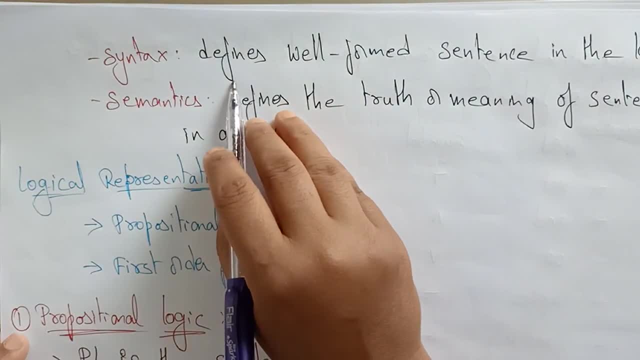 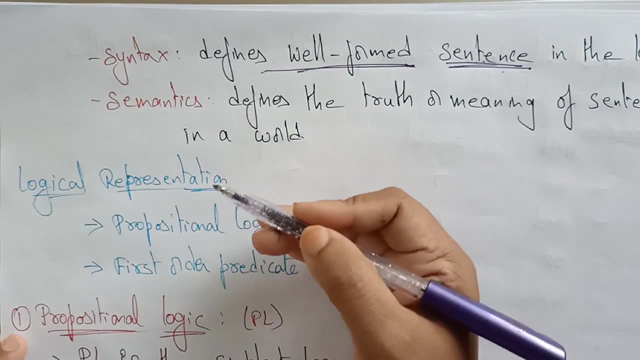 what is a syntax and what is a semantics? A syntax is defined as a well-formed sentence. in the language It's just a well-formed sentence. Then what is a semantics? Semantics defines the truth or meaning of the sentence. So, whatever the syntax that is represented in the 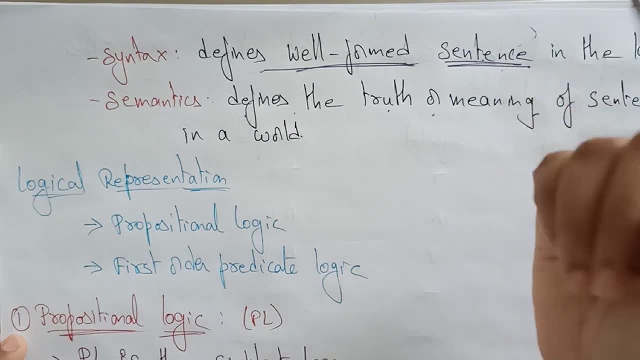 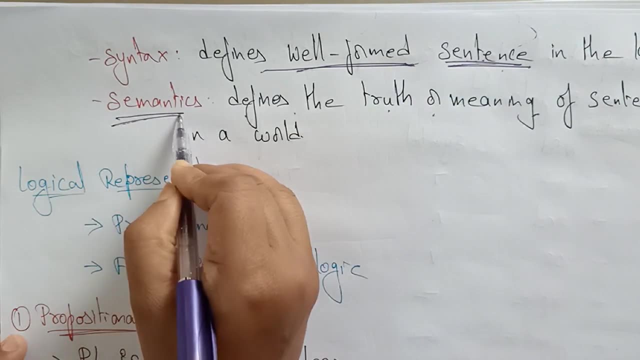 form of a formal language that defines means, whether it is a true and what is the meaning of that sentence regarding to the world or the environment? That explains about the semantics. Semantics is nothing but the meaning given, whatever the meaning that it is given come from. 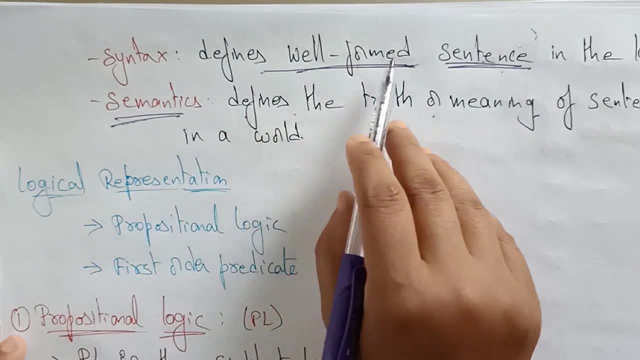 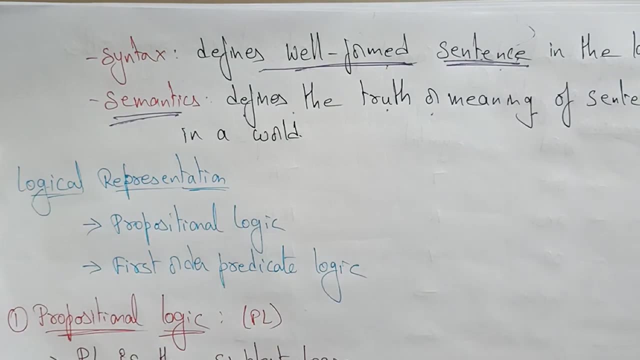 the syntax. A syntax defines a well-formed sentence in the language and semantics defines the truth. Okay, so the law I said I am going to explain about the logical representation. So the logical representations can be explained with the help of propositional logic or the first order predicate. logic means proportional. 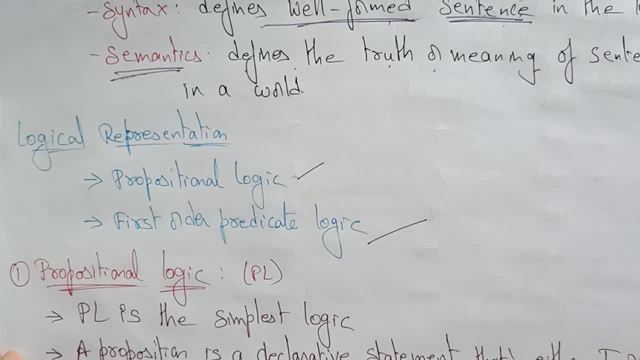 logic and the predicate logic. Now let's see what is this? propositional logic. Okay, so we are talking about this. logical representation means one of the technique of knowledge representation. One of the technique of the knowledge representation is the logical representation. So in that I'm taking as the 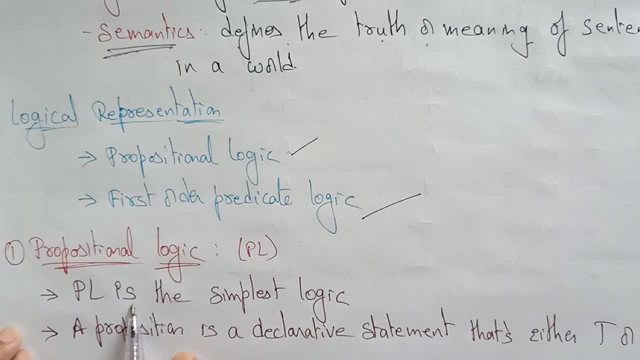 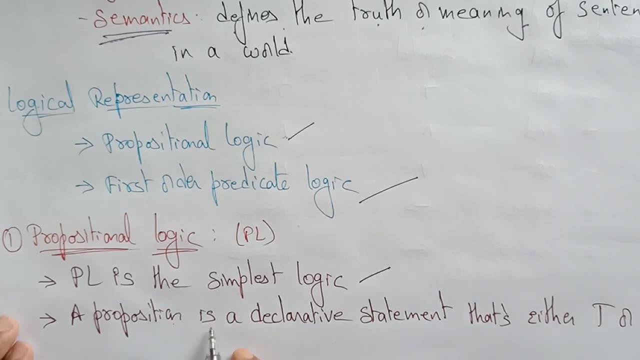 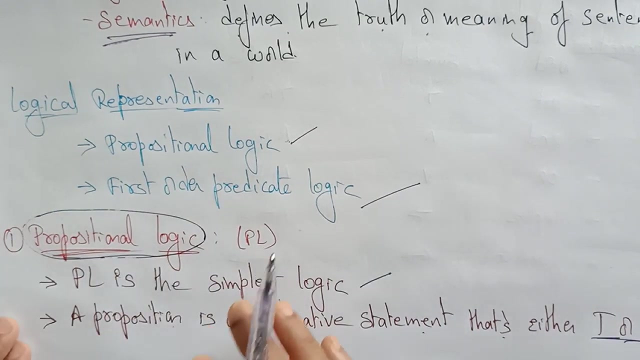 with propositional logic. a propositional logic is the simplest logic. so when compared to all the logics, the propositional logic is the simplest logic. a proposition is a declarative statement. that's either true or a false means. simply, it is a declarative statement. it can do or die. 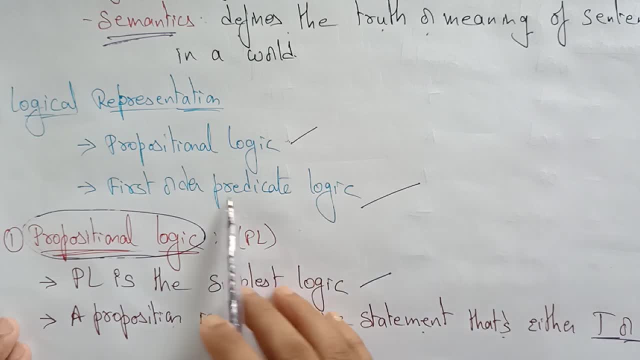 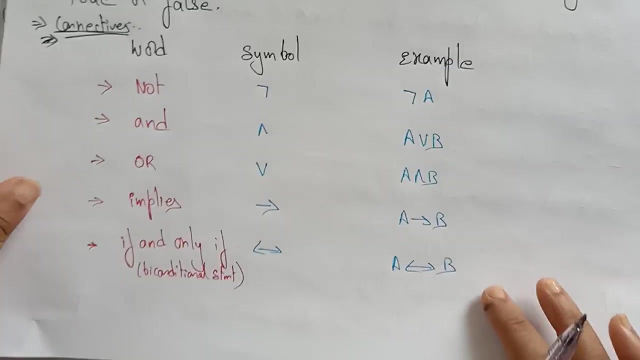 do or die, just is true or false, whereas predicate logic- mean we it- is in somewhat a confusion state. it is just predicating, okay assuming, but whereas propositional logic will not assume. it's just a declarative statement. either it can true or it can false. so that they are explained. 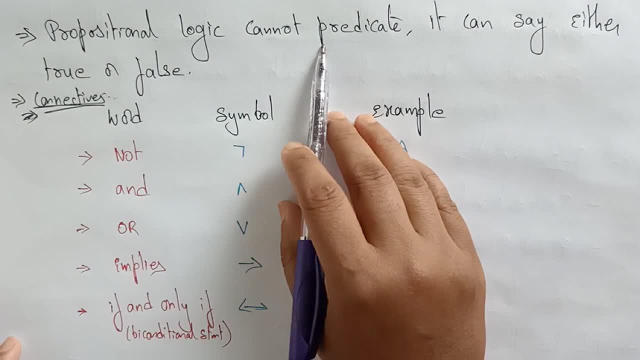 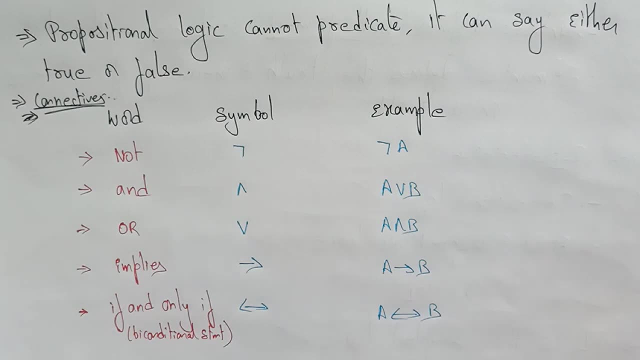 the propositional logic cannot predict, it cannot predicate, it cannot assume, it can say either true or false because it is declarative. so the connectives that are used in the propositional logic, so let's see what are the symbols, that connectives that we use in the propositional 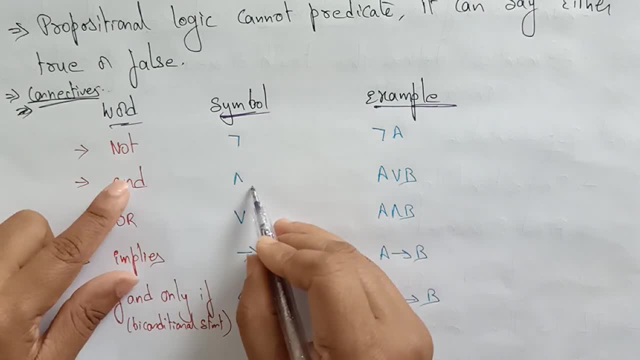 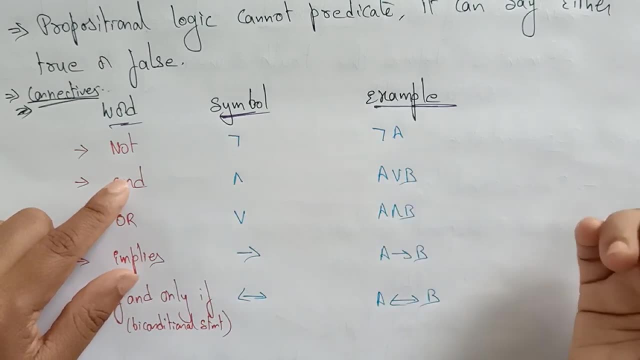 logic. so this is a symbol of the not and this is for, and i think you already know about these propositional logics, okay, you will learn in the discrete mathematics also, okay, and the theory of computation. so all the subjects you, uh, those subjects, you learned about these connectivities. 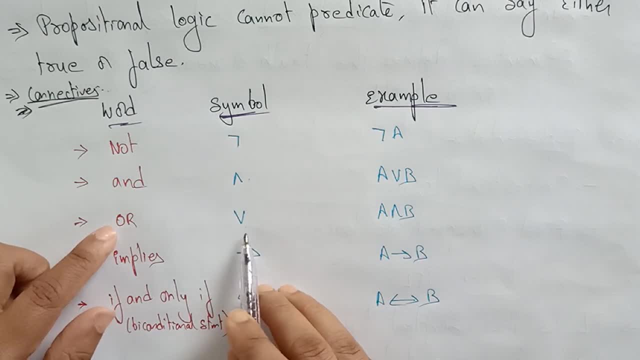 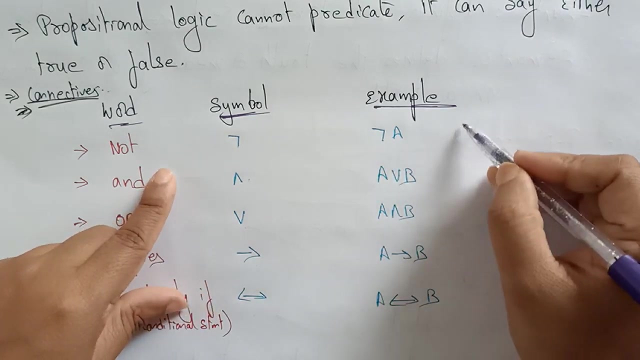 this is a symbol of and and this is or. and this symbol implies: it's nothing but implies, and this is if and only if, which we call it as a bidirectional statement. so example, let's take: not a means a, b or the two sentence here. not A means just the opposite of A, whatever the A they're. 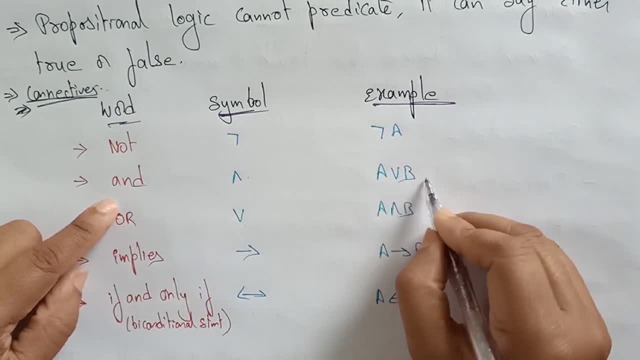 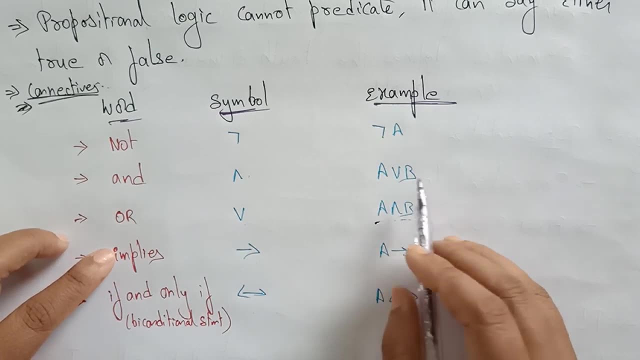 given. just, it's simply opposite of E is a or B I. if either a are B, a and b, the boat should be true here. either one of the things should be two. hey, in practical as if, and only it's going to. Okay, I'll explain this: the girl to the two tables. 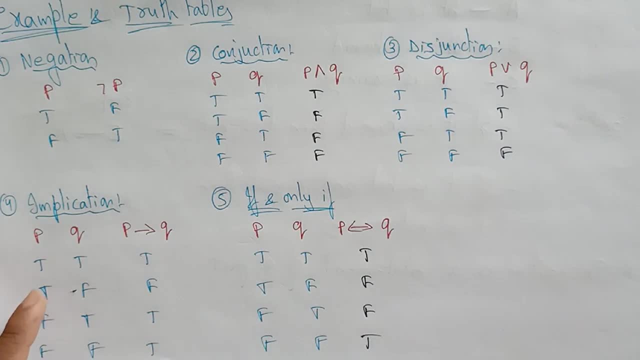 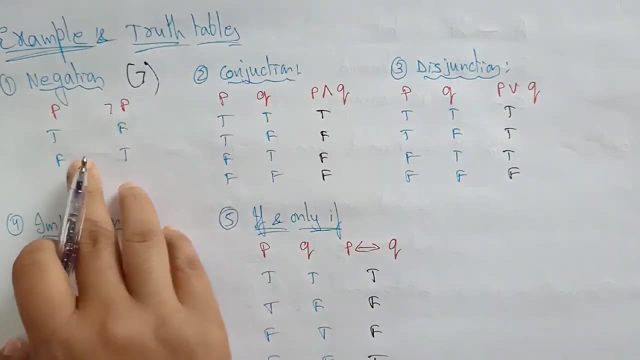 Let's see We are talking about it. will it? will B, please, with the help of the truth tables? Okay, let's about the prepositional logic. So let's see the example and the truth table of this prepositional logic. I said this is a negation symbol, right? These are all the connectivities. Suppose P is 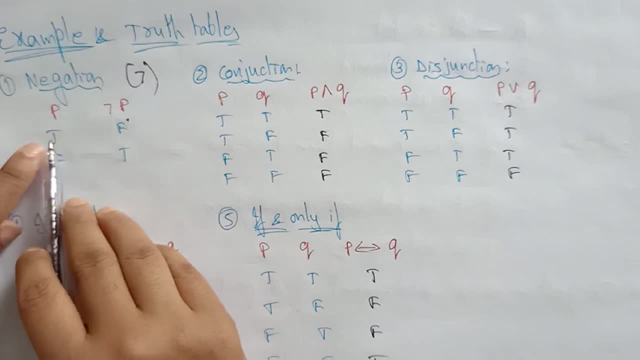 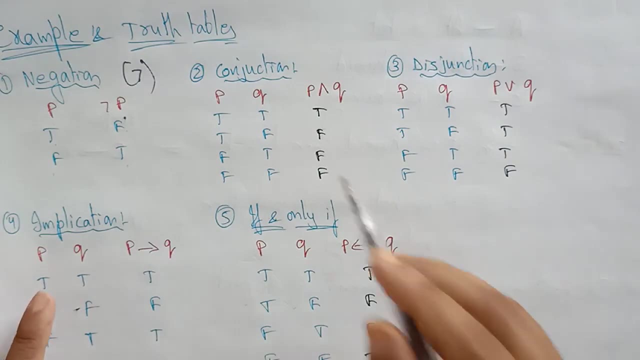 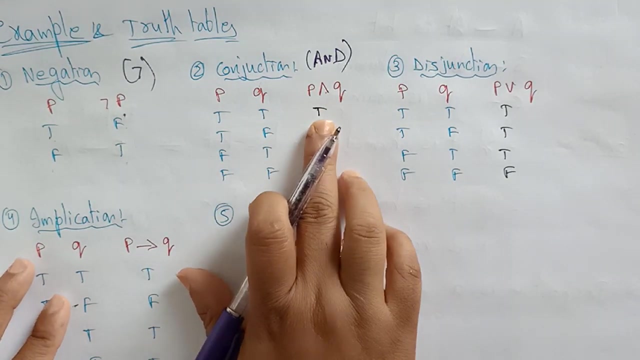 a statement and negate P. So when the statement is true, then the opposite is. the negate P Means it will be false. Whenever the false is there, negate P is true. Now coming to the conjunction. Conjunction is nothing but the end symbol. End symbol: is the conjunction True? true, then only. 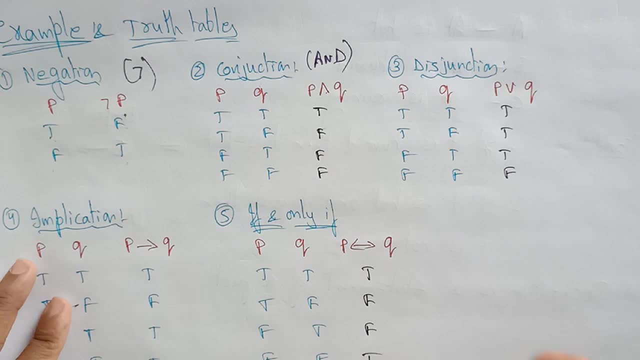 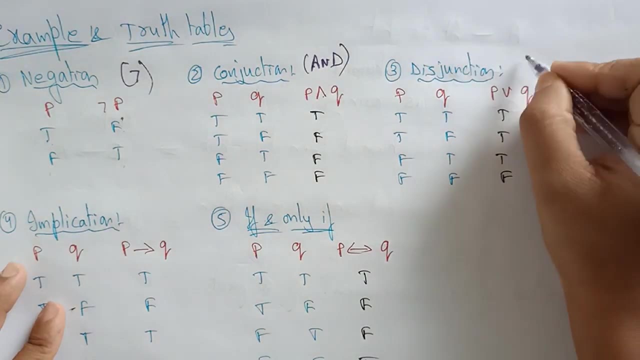 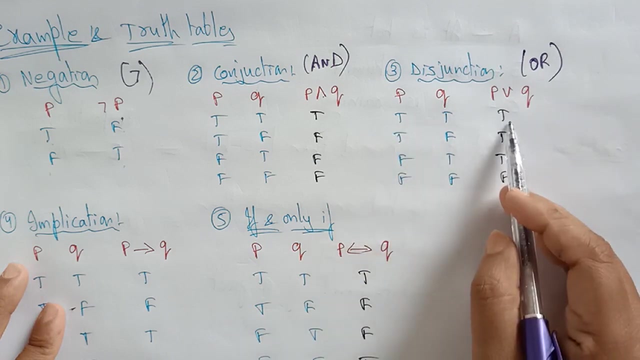 true and the remaining all should be false. When P and Q, both the statements are true, then only P and Q should be true. Otherwise the statement is the false. Now disjunction, Disjunction is represented as or Whenever. any one of the statement is true, then PRQ will be true. If 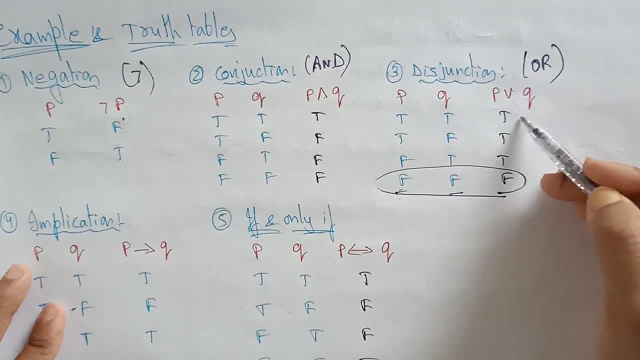 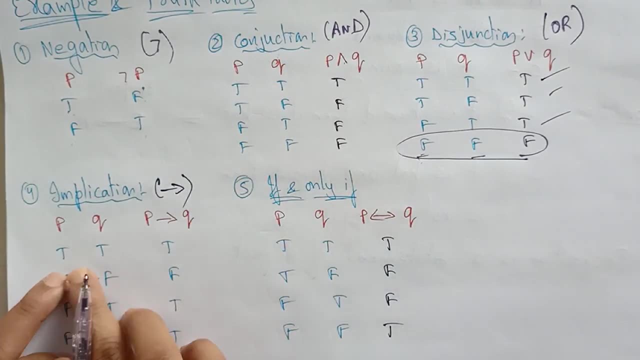 both: the statement is false means then only it will be false and the rest of the things will be true. And coming to the implication, So implication symbol: Whenever the statement P is true, then Q is false. Obviously the P implies Q should be false. okay, And the rest? 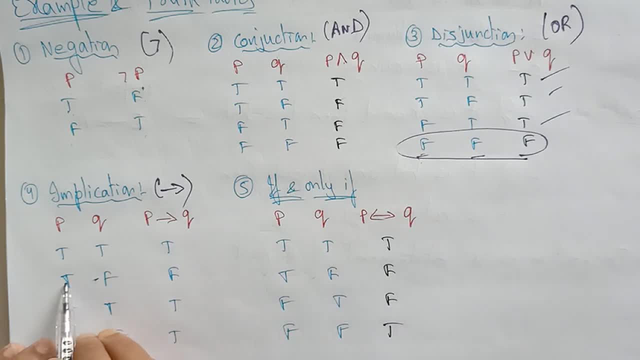 of the statements. it is true Means either. suppose P is false, Q is false, then P implies Q is true. If P is true, Q is true, it will be true. Suppose P is true, then P implies Q is true. 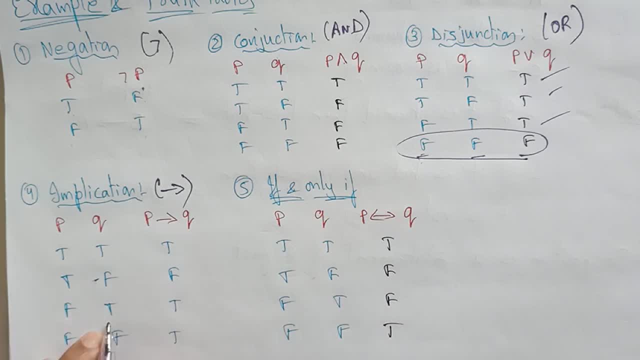 Suppose P is true, Q is true, it will be true. Suppose P is true, Q is true, it will be true. false: the statement: first statement is false and the second statement is true. obviously it takes the second statement okay, whatever it is there in the second statement if second statement is. 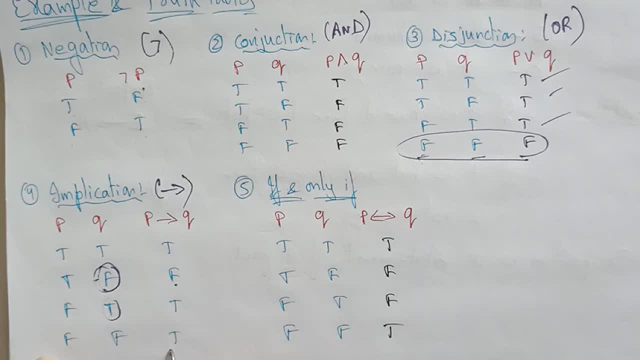 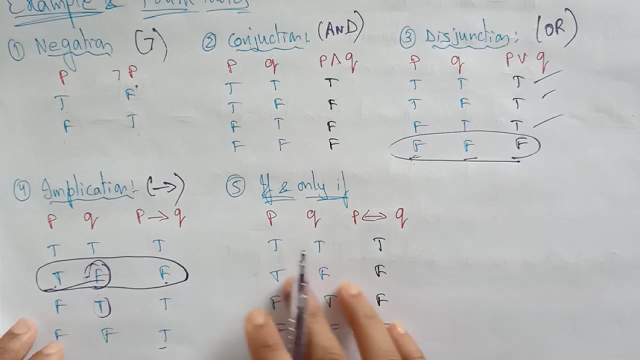 false, it will be false. if both are the false means it takes true only the thing, this thing you have to be remember that whenever the second statement is false, when the first statement is true, it implies false. and if, and only if, means both should be the same. if true, true, is that true. 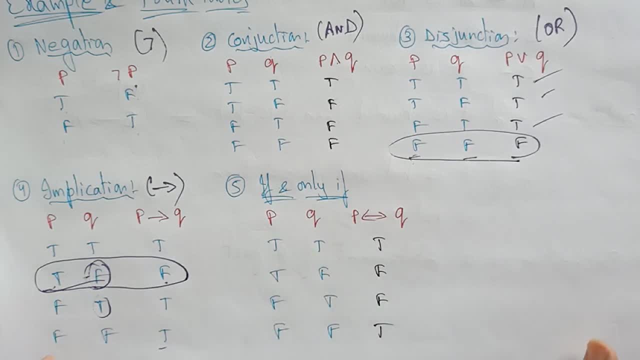 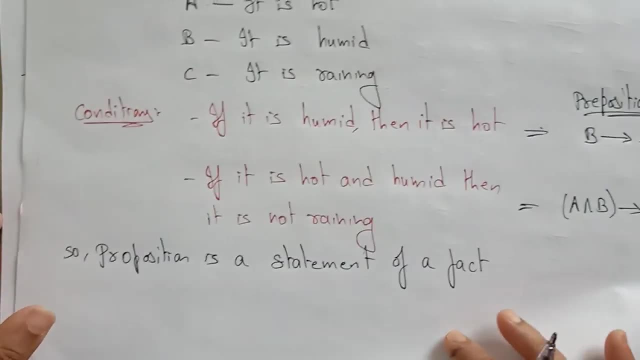 and false. false is their truth, then the remaining things will be false. that is a bi-directional statement. so these are the true tables of the propositional logic. okay, now let me take a simple example to explain this propositional logic. i have taken a statements here a. i have taken a. 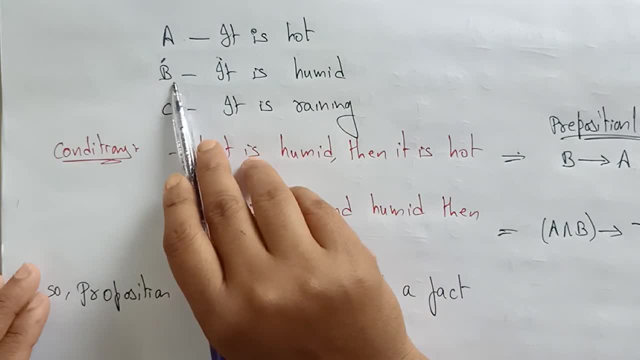 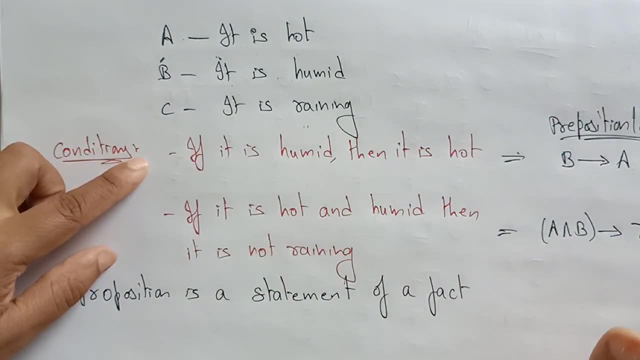 statement a is it is hot, it is a statement, and b is it is humidity. whenever the c is there, it is raining. now let's see some conditions and i'll write the prepositional logics in the terms: uh, in this, with the help of the prepositional logic, i will write the prepositional logics in the terms: 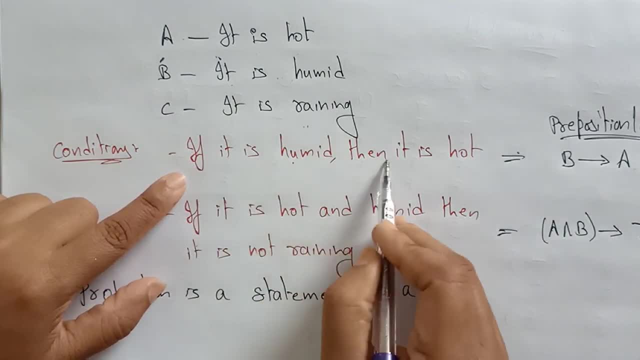 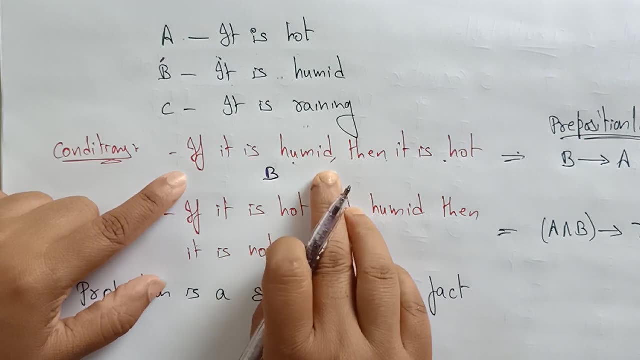 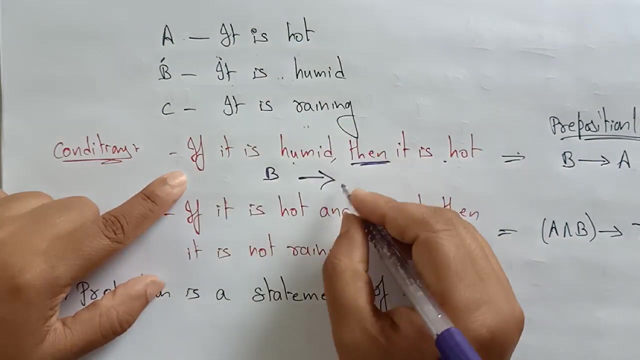 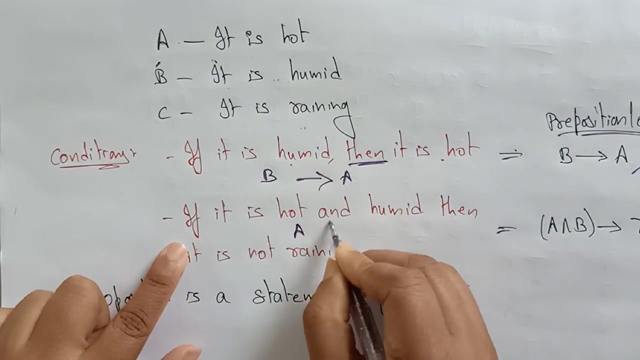 of the connectivities. if it is humid, then it is hot. if it is humid means b- okay, if it is humid means b, then it is hot. then means then is represented by: implies it is humid, then it is hot. b implies a second statement: if it is hot means a and and symbol and is represented like this: okay and humid. 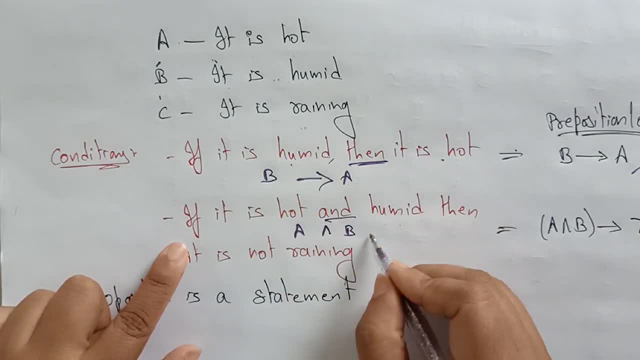 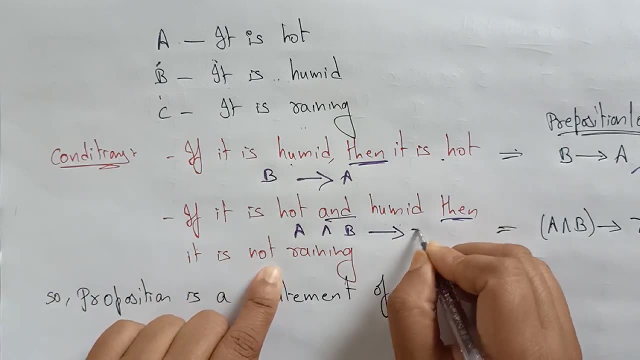 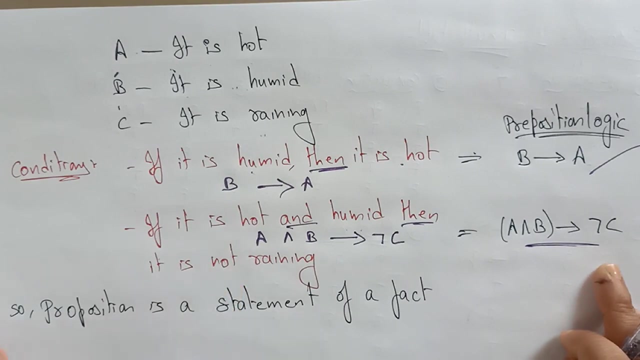 and humid means b. if it is hot and humid, then then is nothing but implies then it is not raining. it is not raining not means. this is a negation symbol. raining is c, so that you got a and b implies negate c. so this is a? uh example of the propositional logic. so, whatever the 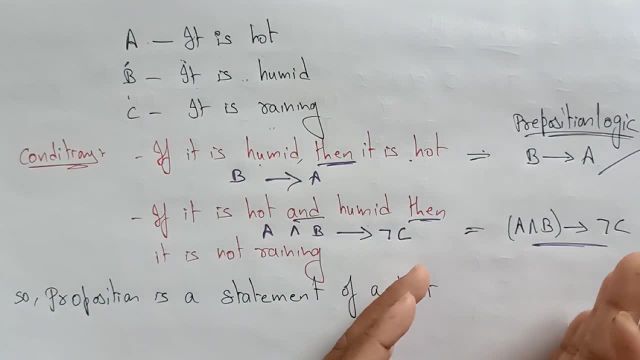 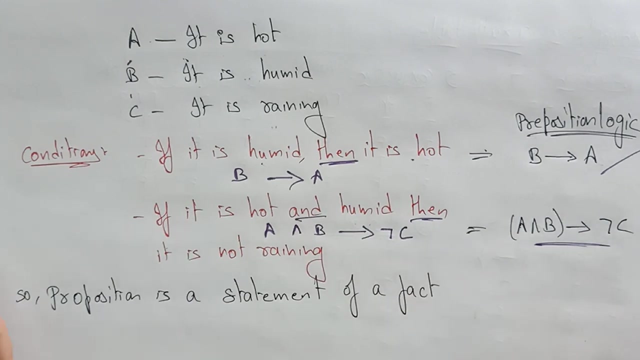 conditions they are given that i represented in the form of a uh syntax. okay, it's a language of the prepositional logic language by using the connectivities. so by this, what we understand? a proposition is a statement of a fact. either it can be true or a false. okay, now let's see some. 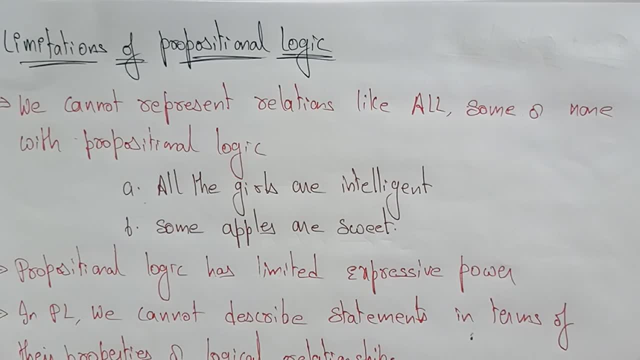 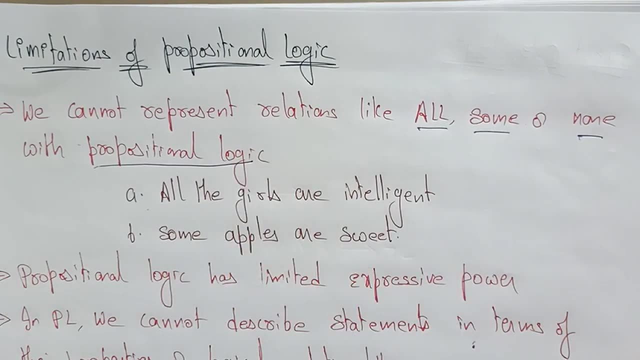 limitations of this propositional logic limitations. we cannot represent, uh, represent relations like all, some or none with propositional logic. so with the uh, the prep, with propositional logics, we cannot use these type of relations. okay, so that is one of the drawbacks of the prepositional logic language. 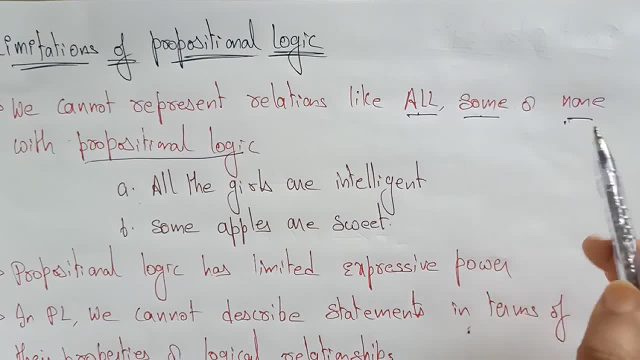 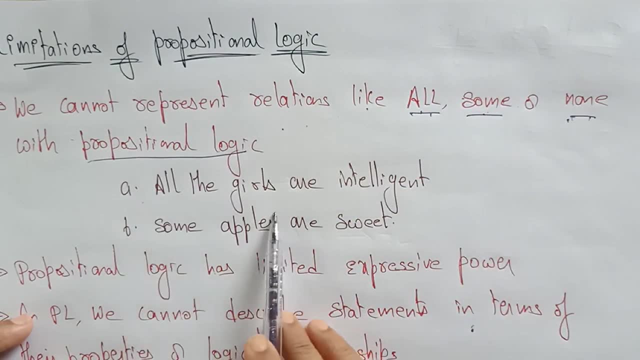 back here. here we are using either true or false, that's it okay, but here, uh, it cannot represent the relations like all some or none, that means uh. these are the examples which cannot represent with the prepositional logic. propositional logic: all the girls are intelligence, okay, and some apples. 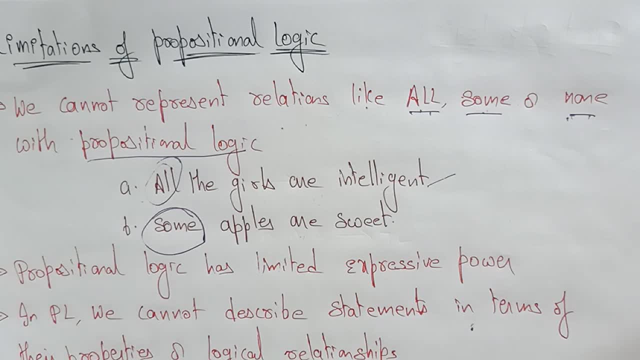 or sweets. here we are saying some apples or sweet, but not it is conformally, we are. it's just a predicating. we are just predicating some apples or, uh, sweet. we are not conforming the statement, we are not declarating, we are not using the declare. these are not declarative statements. that means they.